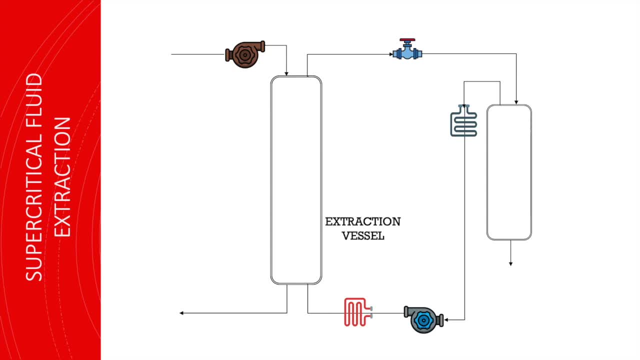 The main unit operation is a continuous countercurrent extraction vessel which provides mixing between the two phases: the slurry feed and carbon dioxide. The slurry feed and supercritical carbon dioxide are continuously and simultaneously pumped into opposite ends of the extractor. The slurry feed and supercritical carbon dioxide are continuously and simultaneously pumped into opposite ends of the extractor. 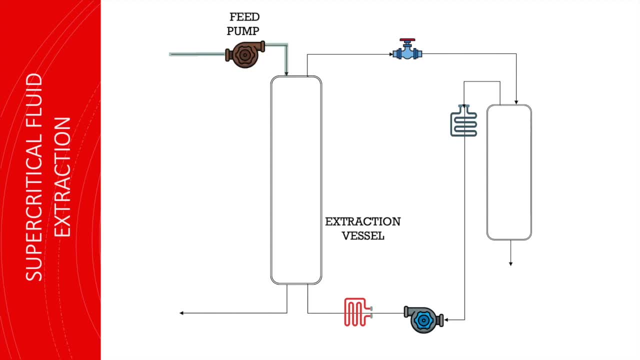 As a result of the mixing in the extractor, the compound of interest from the slurry feed dissolves into the supercritical carbon dioxide. The supercritical carbon dioxide carries the dissolved compound or compounds out of the extraction vessel Continuously, and simultaneously the extract-free slurry feed also exits the extraction vessel, which is an�ild. 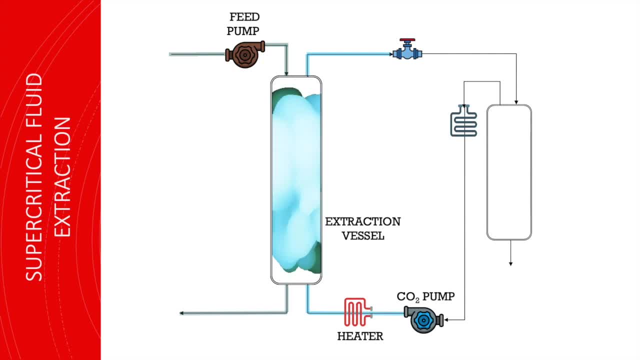 to the free-form slurry feed When the extracellular feed of SCFGAN- violated deep seavaluation using SCFGAN 감사 material. Dieide bijacking by fusion stream. кеinte Thi将 ajейент exits from the extraction vessel the supercritical carbon dioxide and 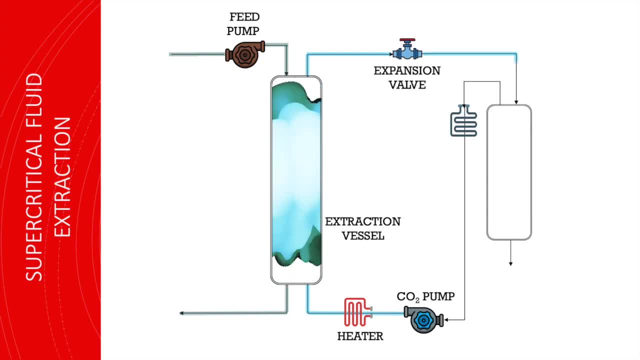 dissolved compound go through an expansion valve where depressurization happens upon entering the separator. as a result of the depressurization in the separator, the carbon dioxide becomes a gas and can no longer hold the dissolved compound. therefore, separation happens between carbon dioxide and the extracted compound. the separated compound, which in most cases is a valuable product, is 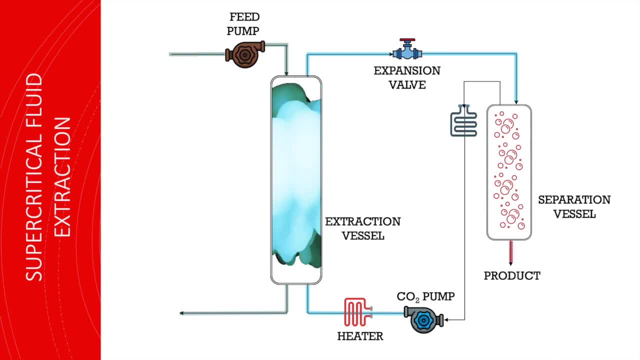 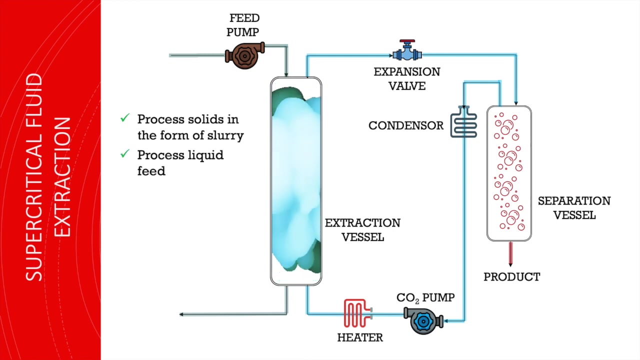 collected from the separator. the carbon dioxide exits the separator and goes through a condenser, where it becomes liquid and is recycled back to the carbon dioxide pump. this fully continuous, supercritical flood extraction process can be used for solids and in the form of slurry and for liquid feed. the process also has the potential. 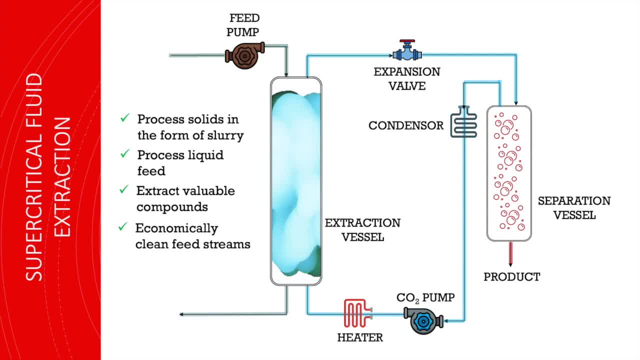 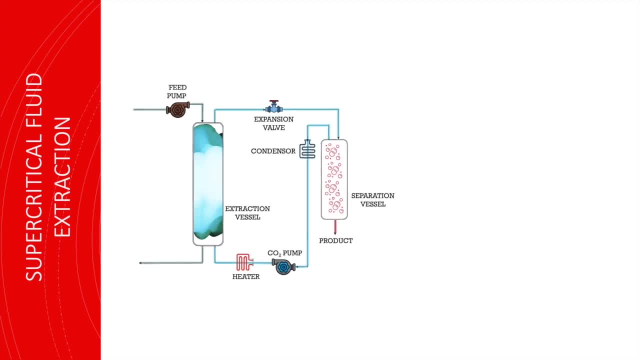 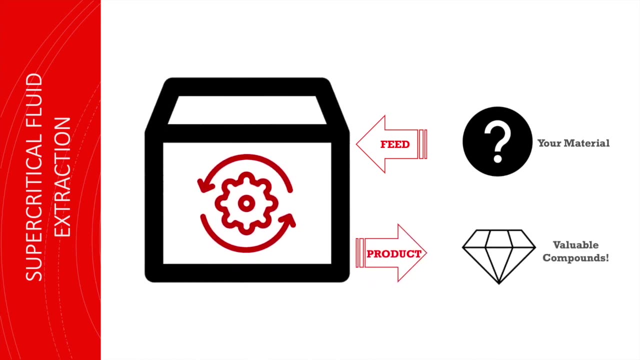 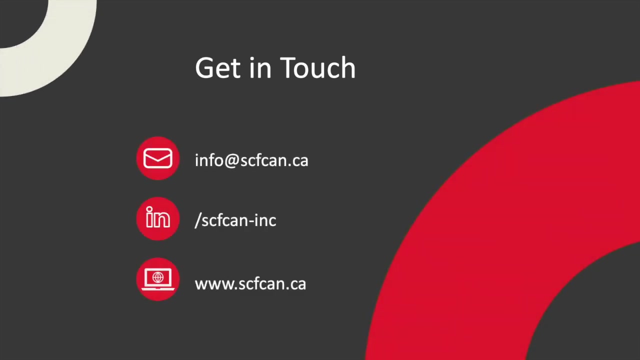 to extract valuable compounds from various feed streams and clean feed streams, both economically and in environmentally friendly manner. is there something you would like to extract? for more information, email us at wwwsfcgovuk. visit our LinkedIn page or our website at scfcanca.